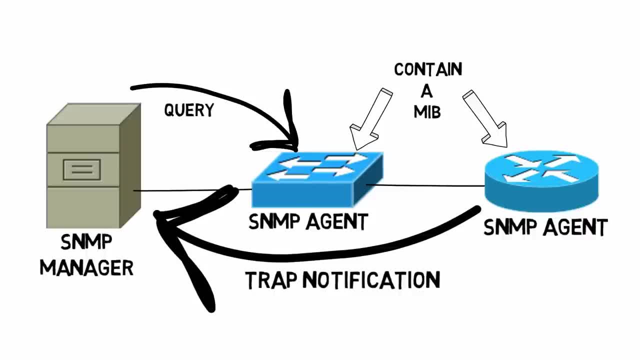 we've talked about thus far. we said that SNMP is made up of really three primary components: An SNMP manager that's going to send queries and receive trap notifications. SNMP agents, the devices being managed. And in each of those SNMP agents we have a MIB, a Management. 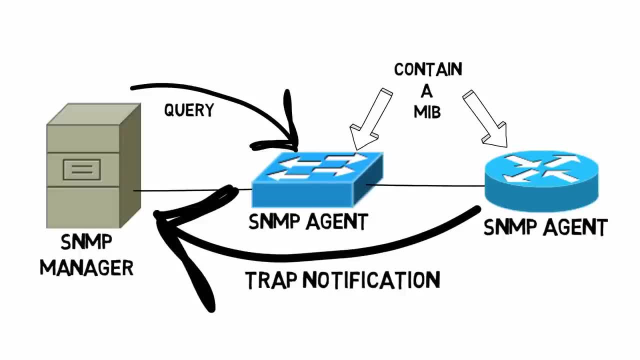 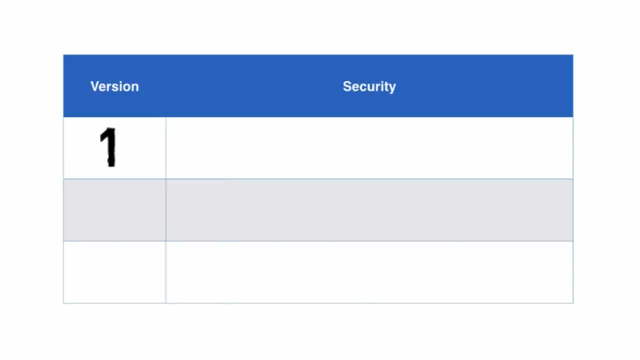 Information Base. And something else we should understand about SNMP is that it's available in different versions. To give you just a bit of a history lesson, when version one came out, the security was not all that great. SNMP devices used community strings which we could think of as passwords, And there 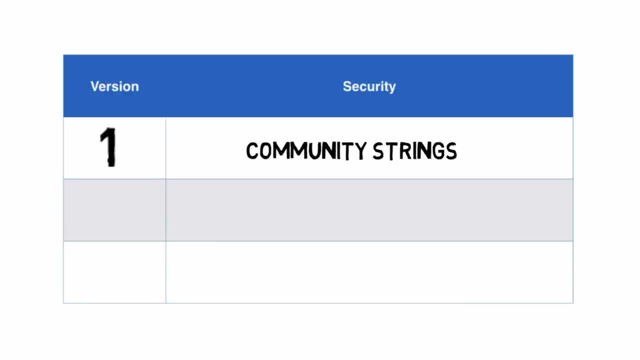 was a read-only community string and there was a read-write community string And if somebody had an SNMP manager and they pointed to a device running SNMP, they could query information from that device if they knew one of these community strings. And if they knew one of these community. 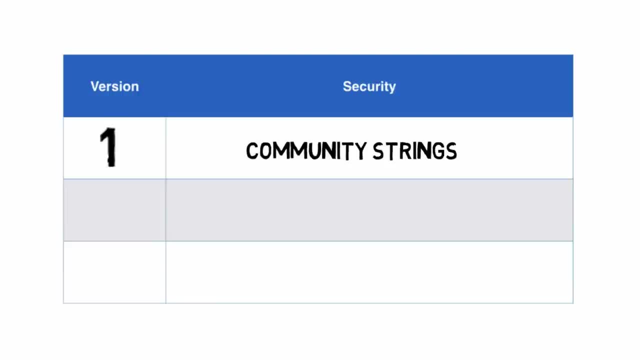 strings. they could query information from that device if they knew one of these community strings. They could read information if they had the read-only community string, or they could even set values if they had a read-write community string. And one of the big challenges that 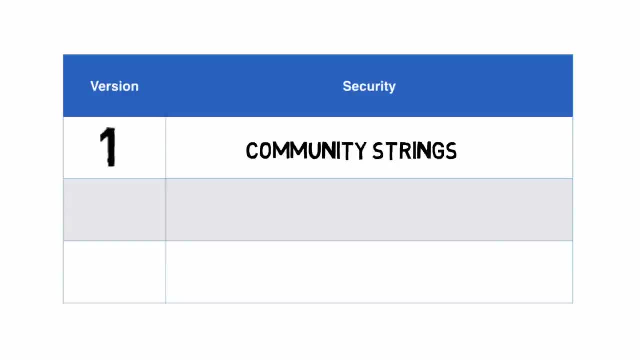 I used to notice back in the 90s. I would get equipment from different vendors and almost all of the vendors had the same default community strings. It was very common for the read-only community string to be public and the read-write community string to be private, And I would 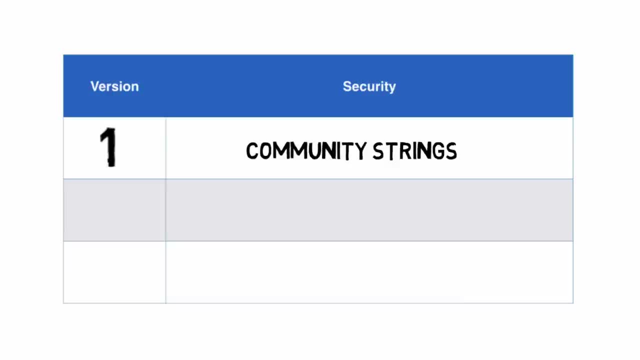 guess that many, many devices got installed in networks that had those default community strings. Not very secure And, interestingly, in version 2 of SNMP security got a lot tighter but it was difficult to set up And as a result version 2 itself never really caught on There. 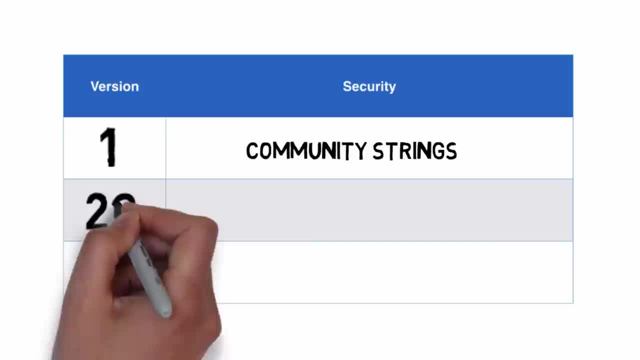 was a variant of version 2 that caught on and that was version 2c, And that's very common in today's networks. And version 2c gave us some of the feature enhancements that version 2 had. For example, version 2 allowed us to retrieve a lot of information from a managed device with a 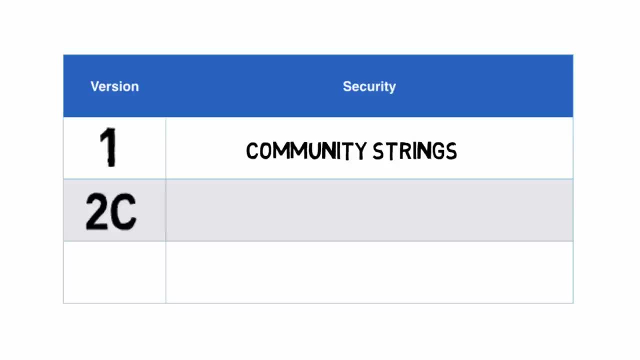 single query and we would need to send fewer queries to get the same amount of information as compared with SNMP version 1.. However, because the security was so complex, the security was rolled back to using- you guessed it- community strings again, And that was version.